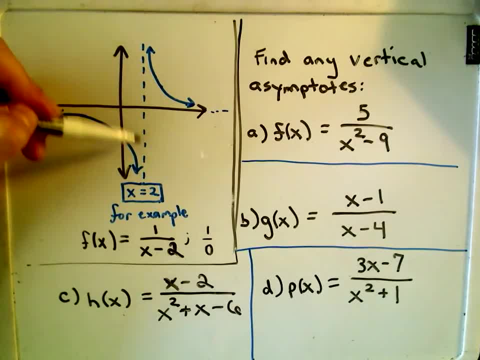 to have a vertical asymptote. So here's the line: x equals 2, we've dashed it. that's going to be our vertical asymptote. And remember a vertical asymptote. all that is is it's an infinite discontinuity. 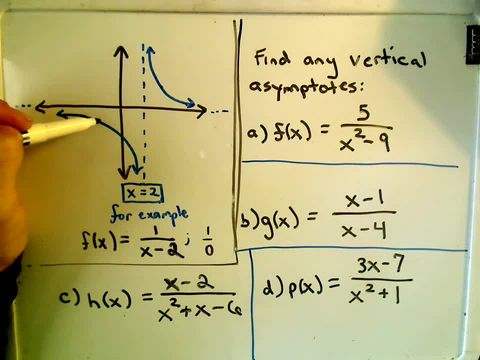 It's the place where the graph is going to be. It's the place where the graph is going to be. It's the place where the graph is going to be. It's the place where the graph either spikes off to negative infinity, you know, it could. 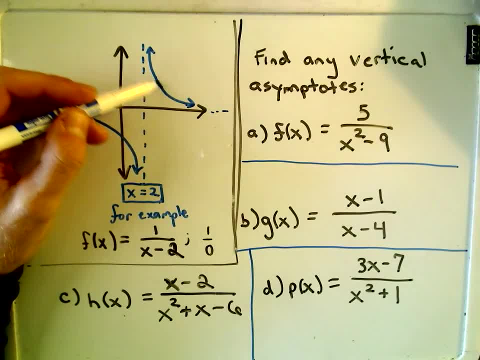 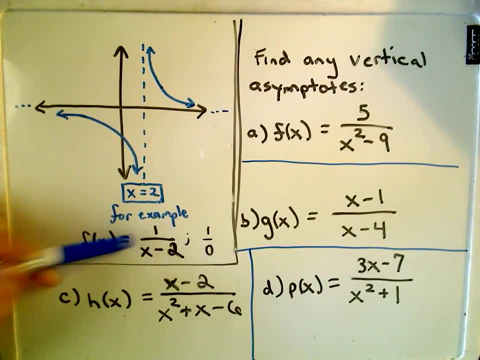 have went to positive infinity. On the right side, this particular graph goes to positive infinity. It could have went to negative infinity as well. It just depends, obviously, on the function that you have. But that's the idea. We're just picking out kind of these places. 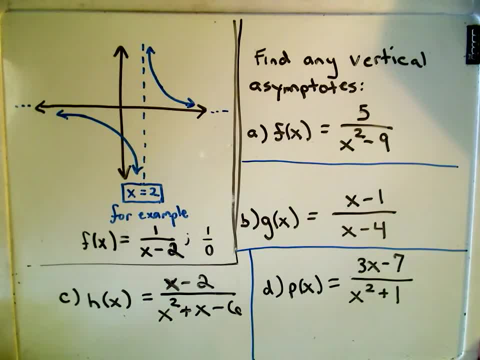 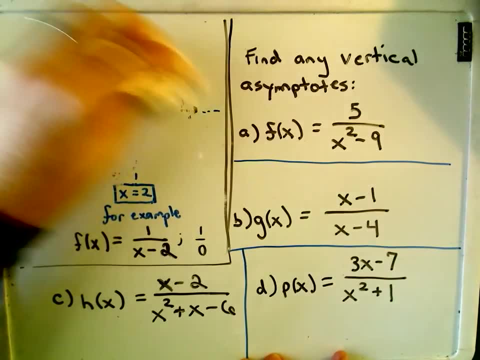 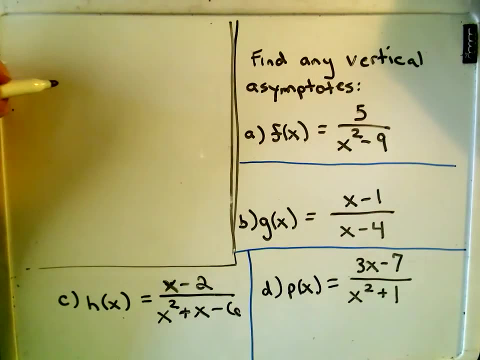 where the graph spikes off to either positive infinity or negative infinity. So here I've got four examples. Let's just find the vertical asymptotes. If there are vertical asymptotes, let's just find the vertical asymptotes for each example. So all I do for these, so maybe 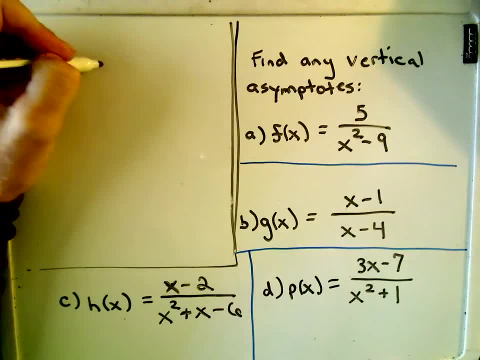 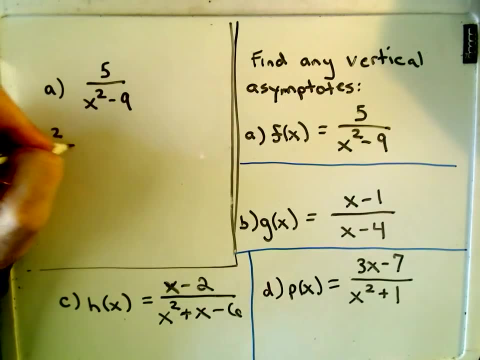 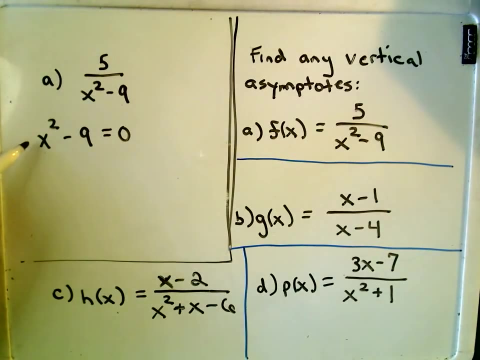 let's look at number. or let's look at a here real quick: 5 over x, squared minus 9.. All I do is first I just set the denominator equal to 0 and solve that. You know, this is going to be the tedious part of finding vertical asymptotes is, you know, depending on what's? 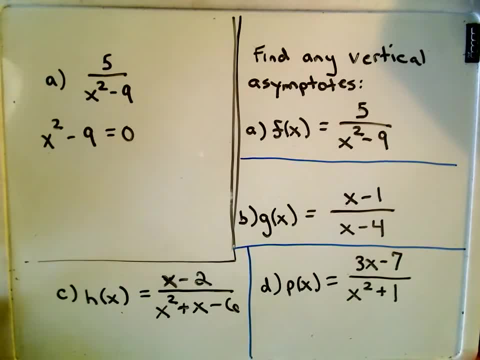 on the denominator. you may have to use different techniques Here. I just have linear equations Or linear functions and quadratics, So they won't be too bad. We could either factor this or we could use the square root property. I could add 9 to both sides. I could take: 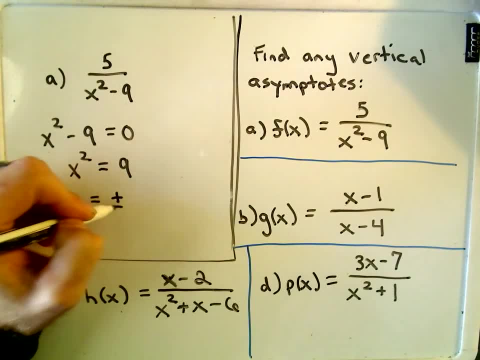 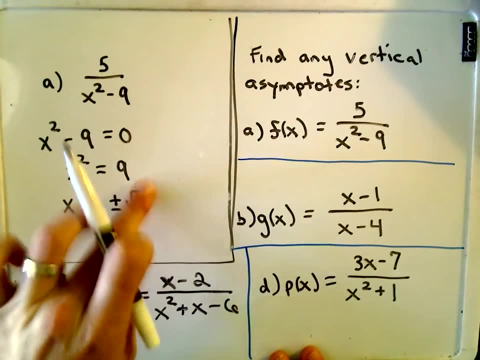 the square root of both sides. But remember, when I take the square root, I have to add on positive and negative. And if you take the square root of 9, well, that's simply going to give us positive and negative 3.. And at this point, to me these are kind of 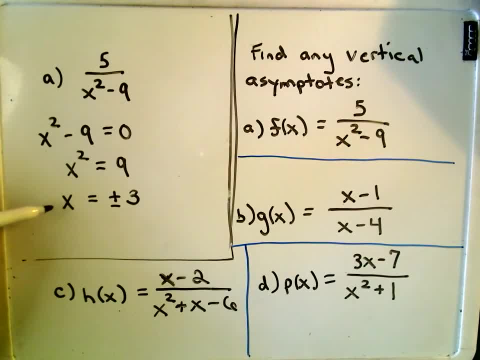 the potential vertical asymptotes. I have to check that if I plug these values of x in, I don't get 0 in the numerator. Well, there's not even any x's in the numerator here, So certainly I'm not going to get 0. 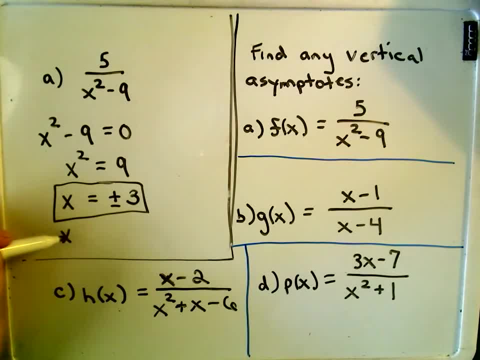 on the top. So these would be my vertical asymptotes. We would have x equals 3 and x equals negative 3 as our vertical asymptotes. Okay, so in a different video too, I'm actually going to graph rational functions, So I don't want to get into the graphing here just yet. 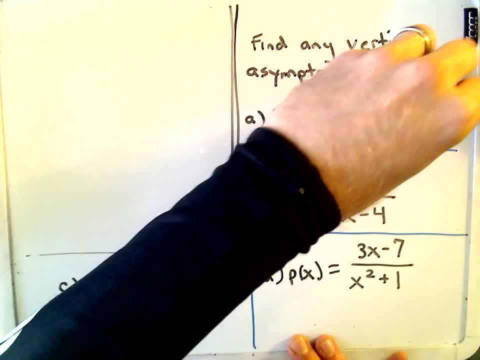 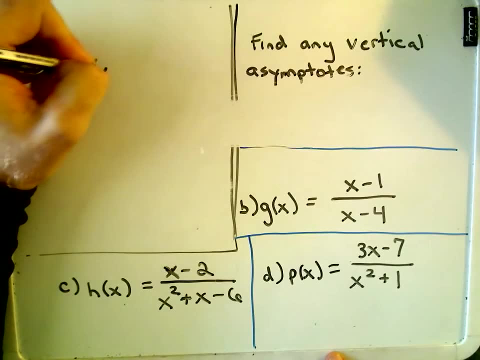 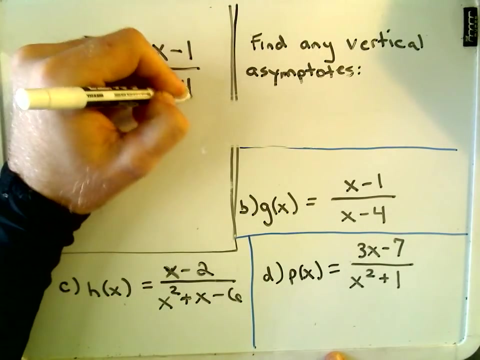 Just talking about how you actually do it. So let's look at the next one. Again, pretty simple examples here, Just trying to give you the idea of what you need to do algebraically. So x minus 1 on top, x minus 4 on the bottom. 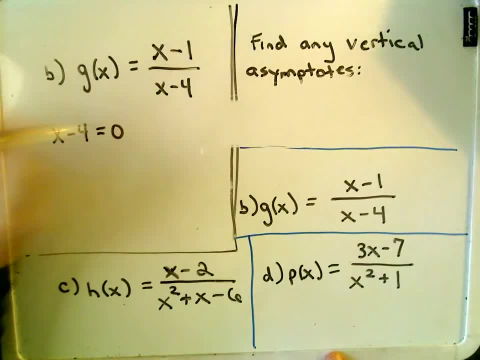 So again, I set the bottom equal to 0. And then I have to solve that corresponding equation Again. here this one's pretty easy, just a linear equation. So all we have to do is add 4 to both sides And we'll get x equals 4.. So again, that's kind of my potential vertical. 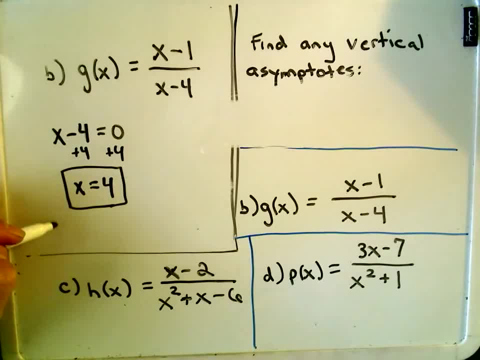 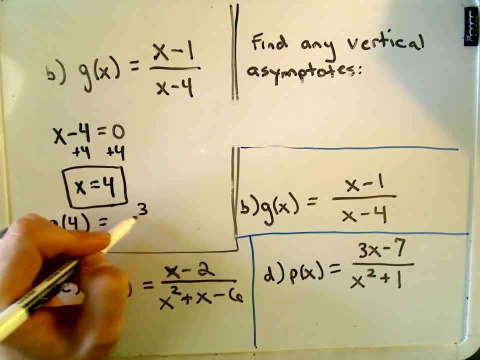 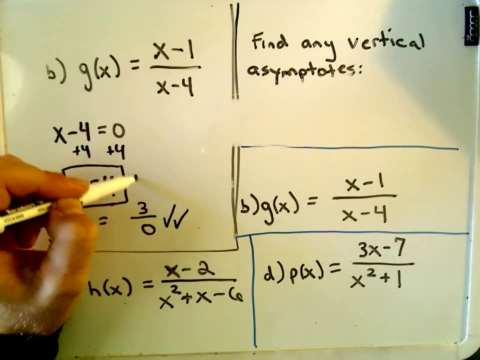 asymptote. Notice, if I plug it back into the original function. if I evaluate g of 4, well, in the numerator we'll get 4 minus 1, which is 3.. On the bottom we get 0. We get something non-zero over 0. That means that this line, x equals 4, is a vertical asymptote. 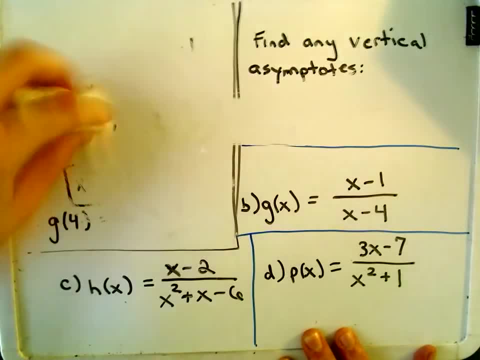 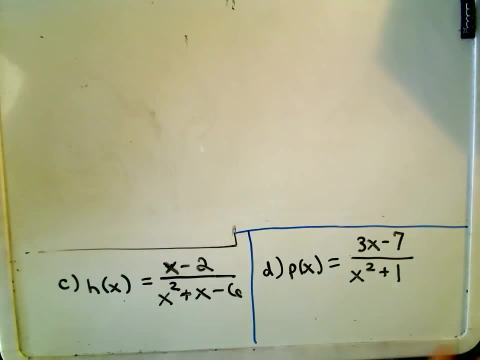 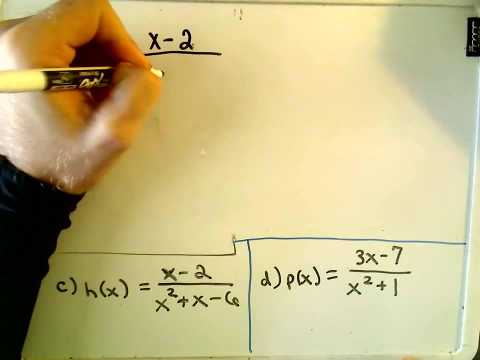 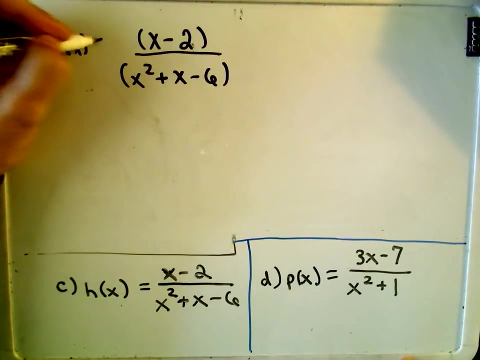 Okay. so let's go to part c here. Okay, same thing. We've got x minus 2 over x squared, plus x minus 6.. Same thing. I'm just going to set the denominator equal to 0 and try to solve that equation. 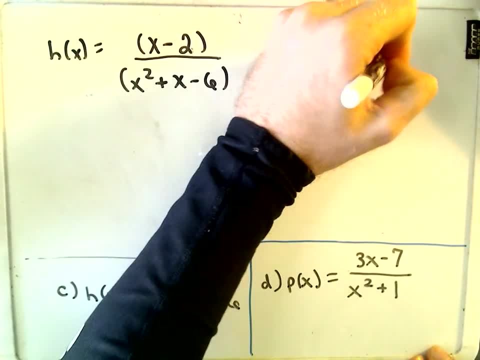 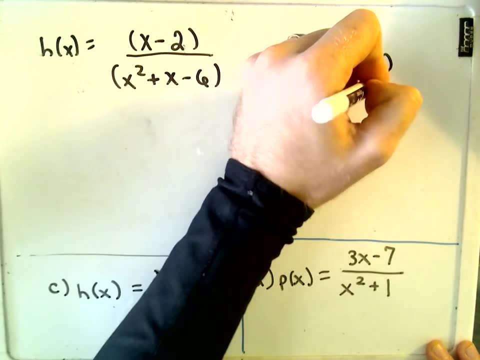 So x squared plus x minus 6.. Thanks, Bye-bye, x minus 6.. Well, again, this is a quadratic. We could use the quadratic formula. I think this factors. So we're going to need an x and an x to get x squared. Remember we need: 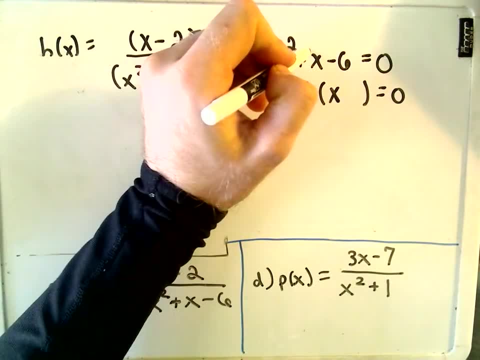 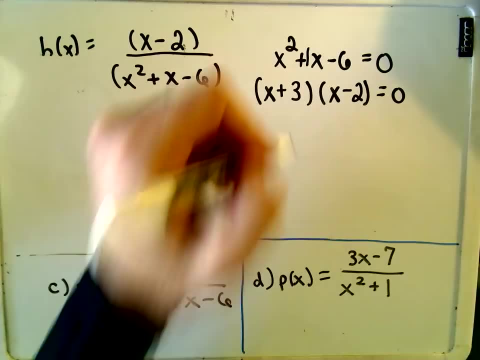 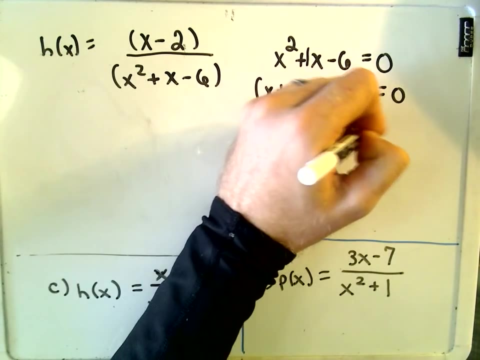 two numbers that multiply to negative, 6, that add up to positive 1.. Well, I think, how about positive 3 and negative 2?? Well, if we set each piece equal to 0, we'll simply get x equals negative 3. And if we set the other piece equal to 0,- the other factor we'll 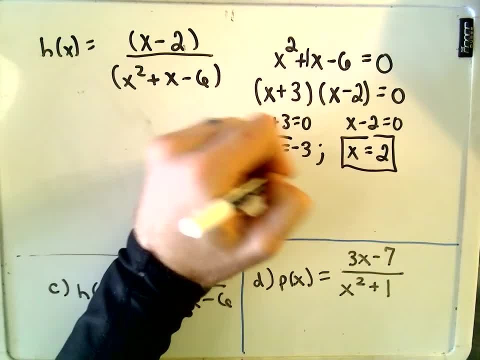 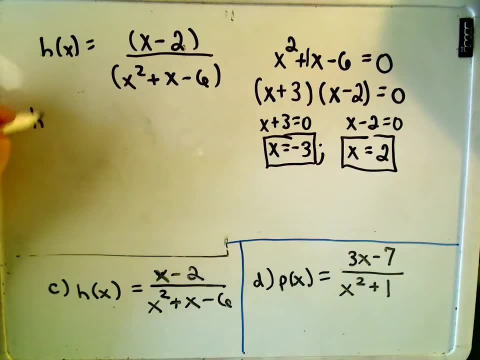 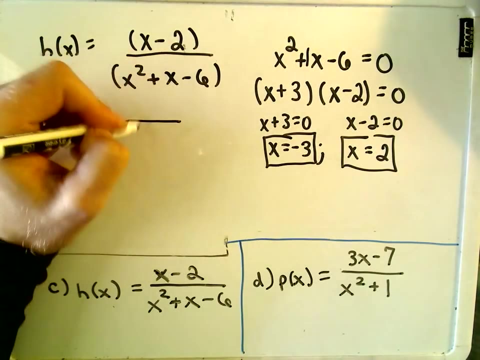 simply get x equals 2.. So these are my potential vertical asymptotes. Again, I need to check and plug each one in Well notice. certainly, if you plug in negative 3, well, on the bottom we said that gives you 0 out. That's what we just solved over there, for If you plug, 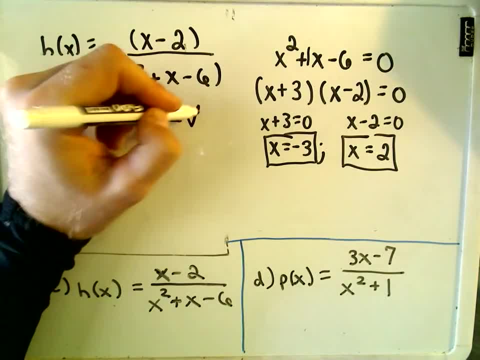 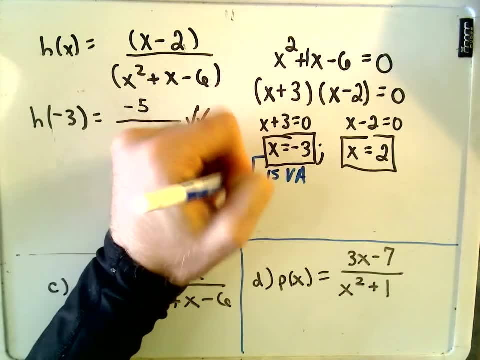 negative 3 into the top, you get negative 5 over 0. That's something non-0 over 0. So x equals negative. 3 is a vertical asymptote. But notice for sure, if you plug in 2 into, 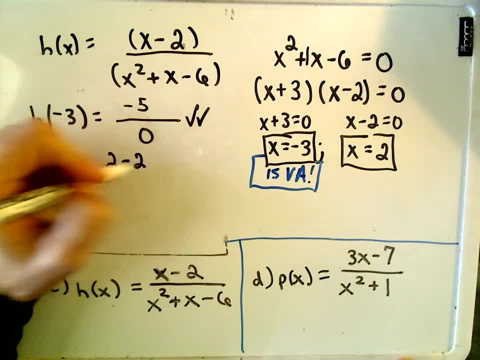 our function. well then, we get 2 minus 2.. Again, we know for sure it gives you 0 on the bottom. That's what we just figured out. Well, here you get 0 over 0. So that means 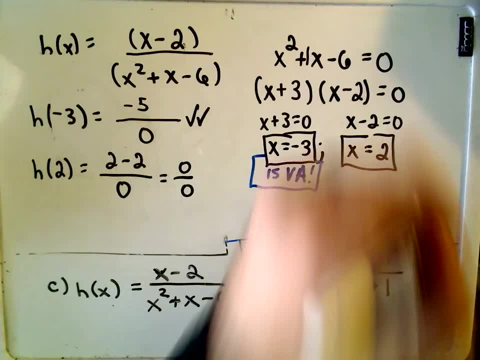 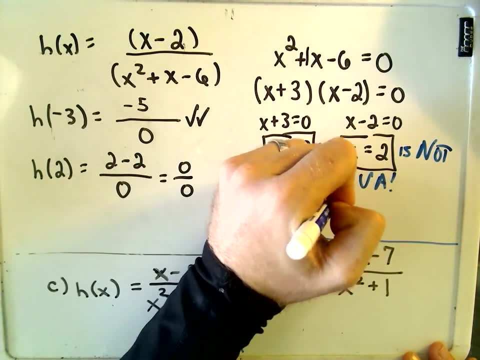 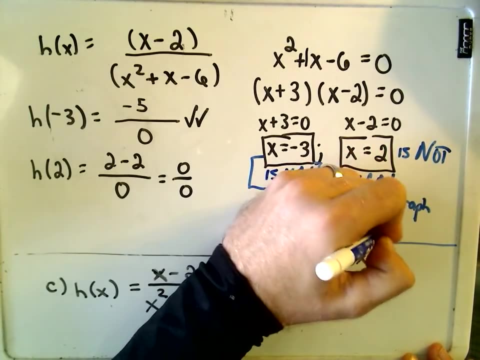 the line associated with x equals 2 is not a vertical asymptote. But again, what it means is you're going to have a hole in the graph at the x coordinate of 2.. That's what's going on if you were to graph it. So again, I think most people they forget to do this. They 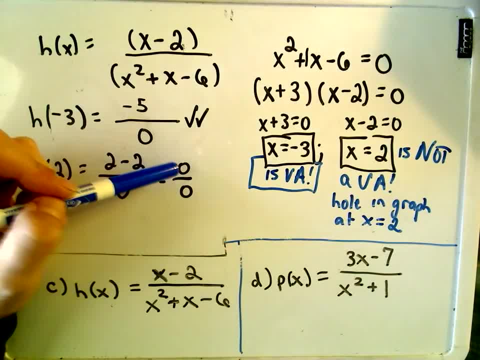 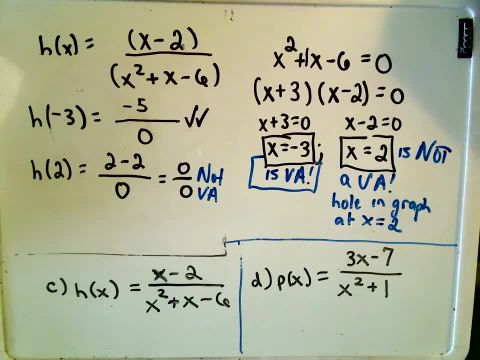 remember it has something to do with the denominator being 0, but they forget to make sure that the numerator is not 0. So for this function, x minus 2 over x squared plus x minus 6, we'll just have one vertical. 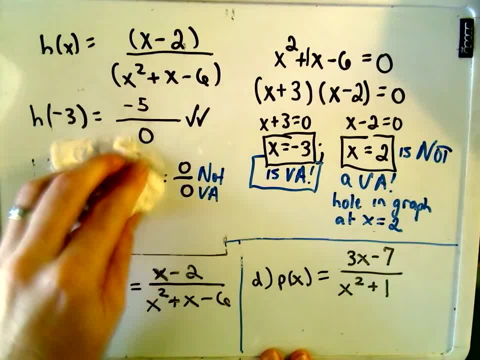 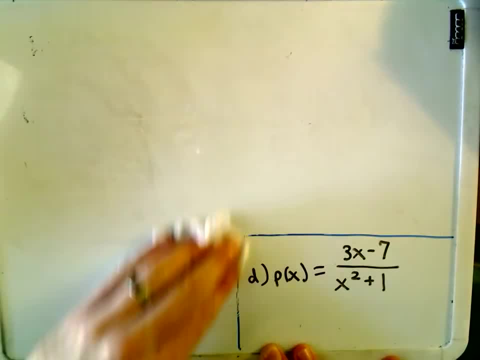 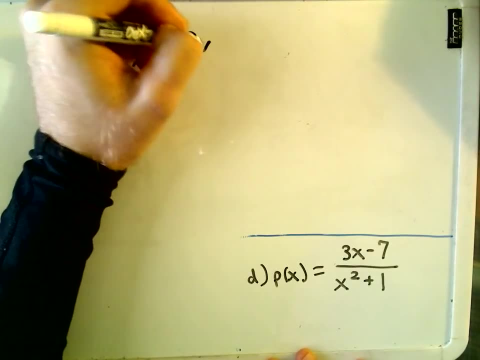 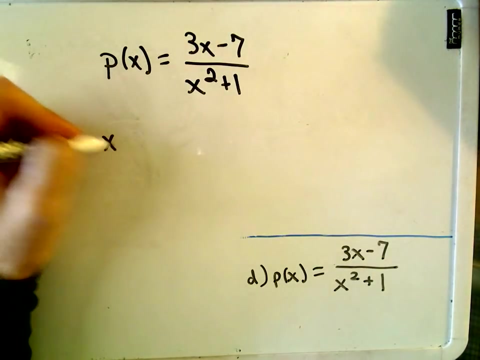 asymptote and one hole in the graph. So, last but not least, let's do our last function here. p of x for Patrick, 3x minus 7 over x squared plus 1.. Well, again I'm trying to find any vertical asymptotes. I set the denominator equal to. 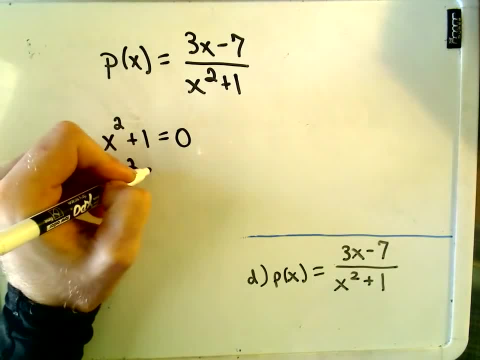 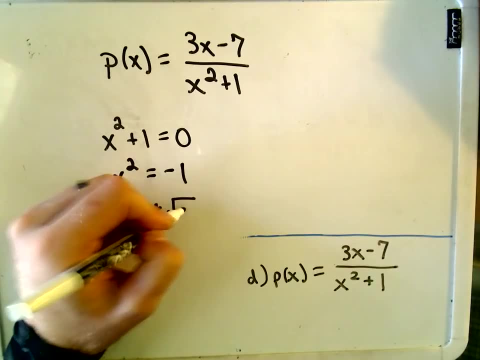 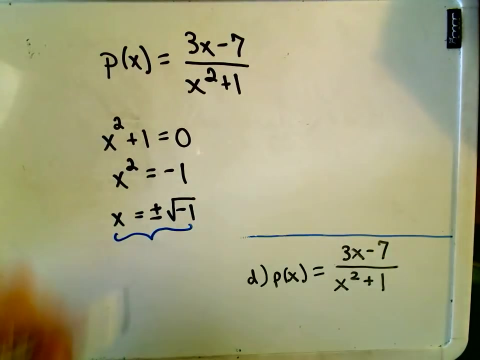 0.. Well, we could use the square root property again and subtract 1 from both sides. But now, if I try to take the square root of a negative number, we could resort to imaginary numbers, but that's not what we want. We're going to use real numbers here. So this is: